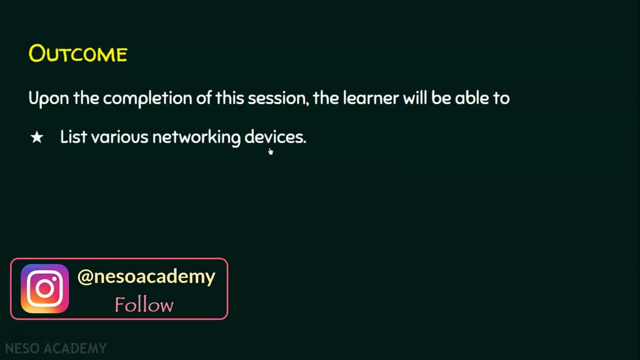 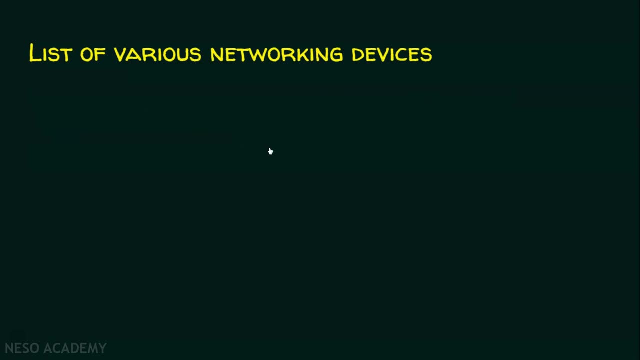 list various networking devices. Let's see what are the various networking devices available. We know there are end devices and intermediary devices or networking devices in a computer network. We have already seen elaborately about end devices. Now we will focus on the various networking devices. 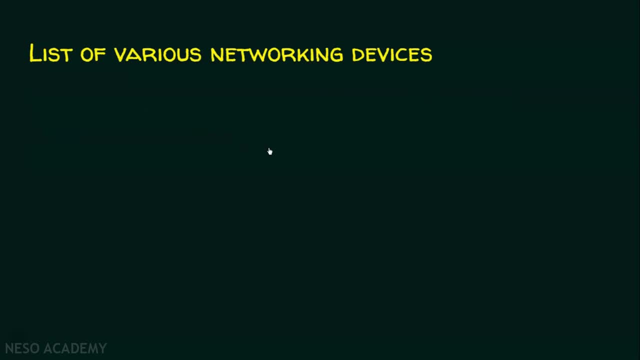 The first networking device that we would like to address is the repeater. A repeater is a layer one device. It means it operates at physical layer. It just regenerates the signal in a single local area network. Second networking device is the hub. 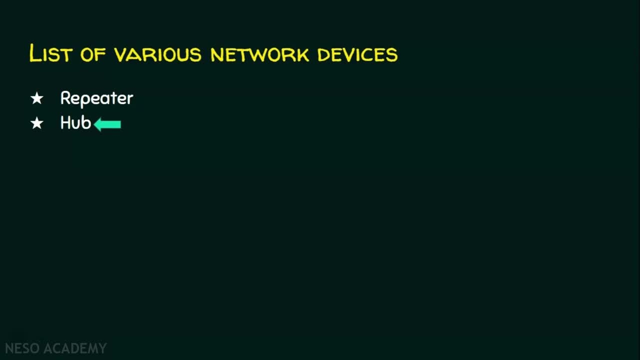 A hub is a local area network device. It operates at physical layer, that is, it is a layer one device and whatever it receives, it always does broadcasting, And that is the drawback of a hub. And coming to the third networking device, which is the switch, 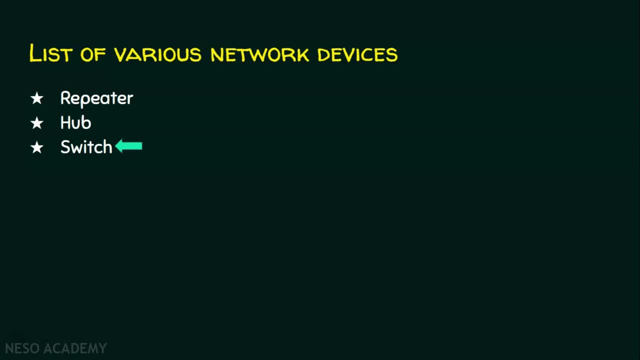 A switch is also a local area networking device and it connects devices in a single local area network. It is a layer two device and it operates at data link. layer Switch is an intelligent device. It stores the MAC address table, Unlike hub switch does unicasting. 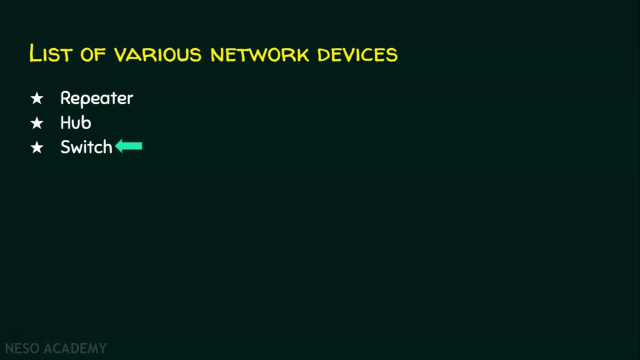 It means it can send the data to the exact recipient, Whereas hub broadcasts the data to all the recipients. And coming to the fourth networking device, which is the bridge, A bridge is also a layer two device. It operates at the data link layer. 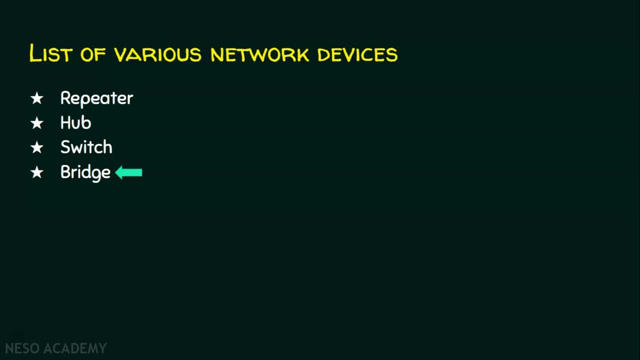 A bridge connects two local area network segments that are running with the same protocols. A bridge can also regenerate the signals, because a bridge is a combination of a repeater and MAC address reading capability. Coming to the next networking device, which is the router. A router is a layer three device. 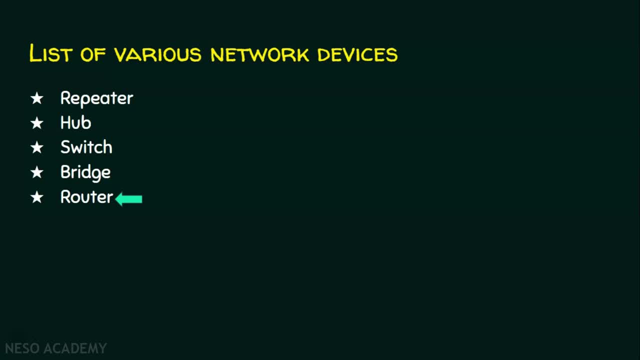 It operates at the network layer. Routers take forwarding decisions based on the network layer. Routers take forwarding decisions based on the network layer. Routers take forwarding decisions based on the network layer. And router is a networking device that can connect two or more different LANs. 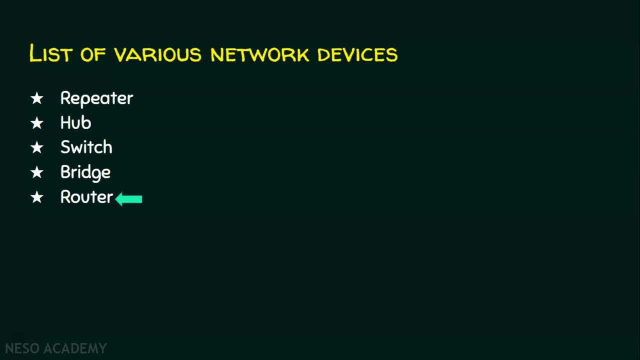 that has two or more different protocols. So one side, if it is ethernet, another side, if it is WiFi and router, can connect these two different technologies as well. And coming to the sixth networking device, which is a multi-layered switch or a layer three switch, 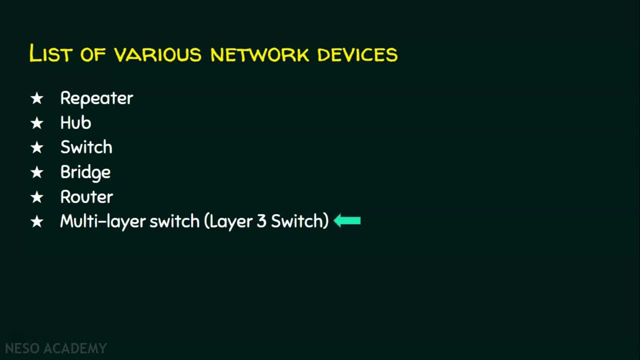 Generally switches are layer two switch. It means it works at the data link layer and it takes forwarding decisions based on MAC addresses, a contemporary switch which is a multi-layer switch. it can be a layer 2 switch as well as layer 3 switch. 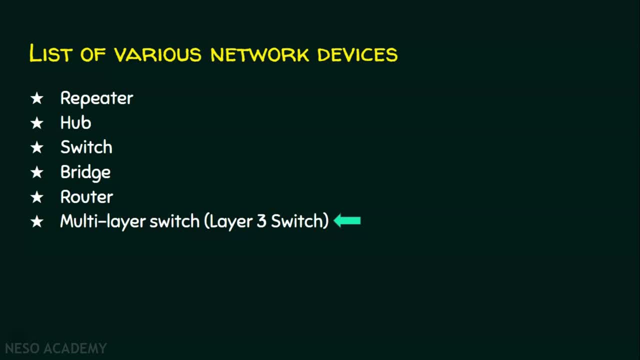 See, it does the functionalities of a switch as well as the functionalities of a router to some extent. So multi-layer switch or a layer 3 switch can act as a router as well as a switch. And coming to the next networking device, which is a Brouter, 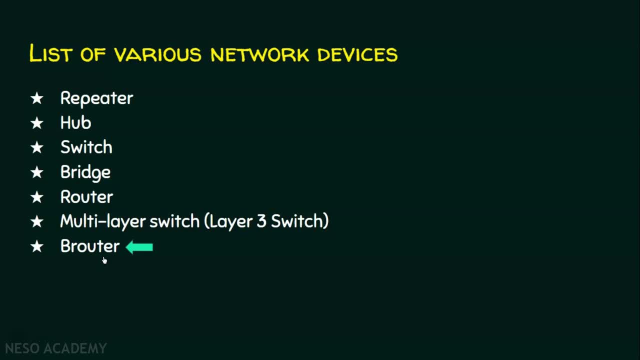 A Brouter is a combination of a bridge as well as a router. A bridge can connect two different LAN segments of same protocol. A router can connect two or more different protocols, But Brouter is a combination of a bridge as well as a router. 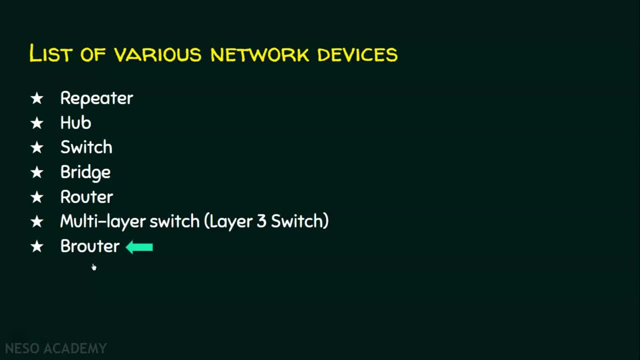 It means it can act as a layer 2 bridge or it can act as a layer 3 router. And coming to the next networking device, it is the Modem. Modem means modulator and demodulator. Modulator means the digital information. 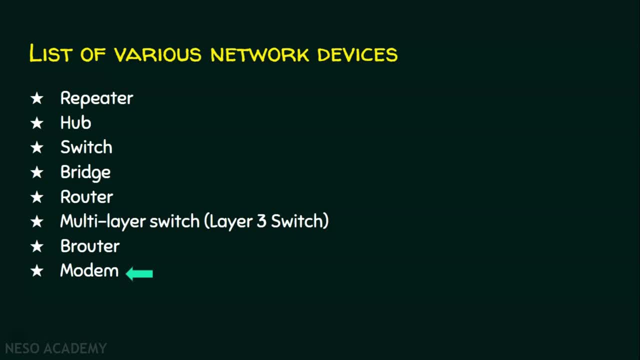 is going to be carried on. a analog carrier signal And demodulator just retrieves the transmitted signal, that is the, the transmitter signal, That is the transmitter digital information, For example, in a traditional landline phones that is exclusively for carrying the voice signals. 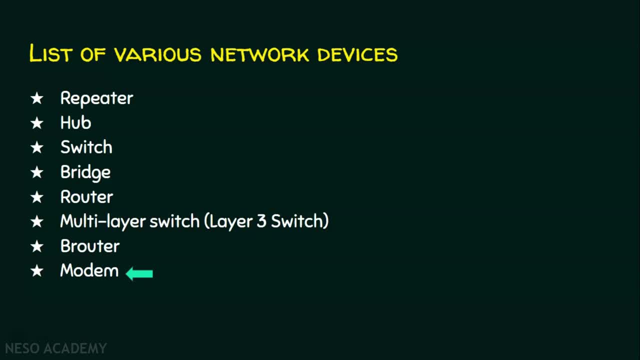 that is, the analog signals, But we can send our digital information using Modem. So Modem does both modulation as well as demodulation tasks. And coming to the last networking device, that is the Firewall, This Firewall is a networking device only. 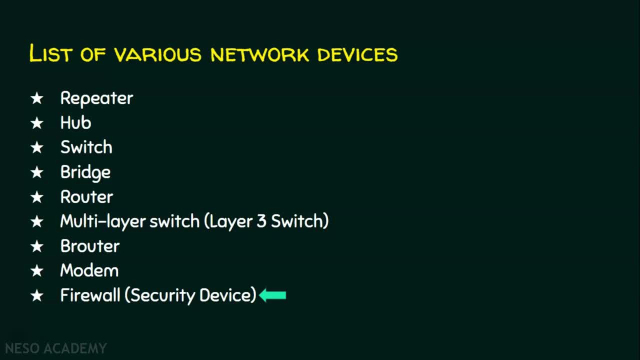 but still it is mainly used for providing security to the network. For example, if we deploy a Firewall in our campus or in our network, this Firewall filters the packet. It filters the packets based on the IP addresses, based on port numbers, based on the application data. 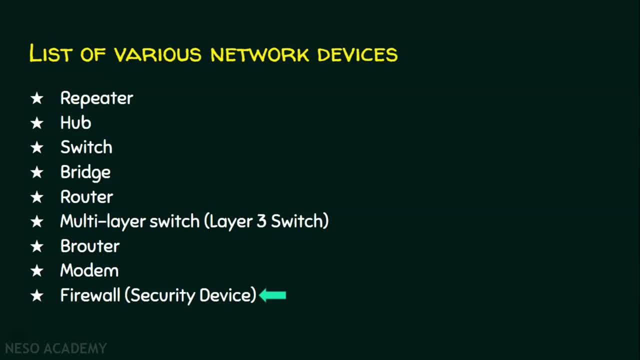 In a network, you don't want any malicious things to happen, So you can protect your network by installing a Firewall. So in a network, a Firewall filters the incoming traffic as well as the outgoing traffic, And that's it. We have listed various network devices.